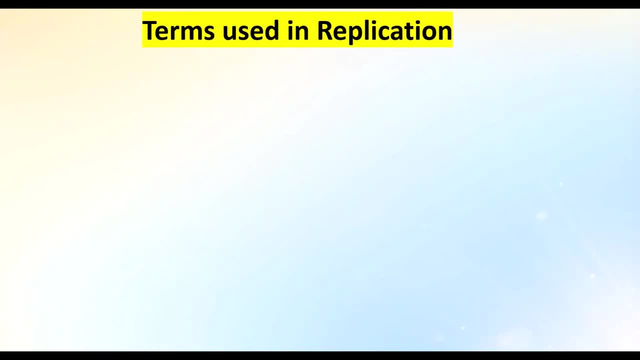 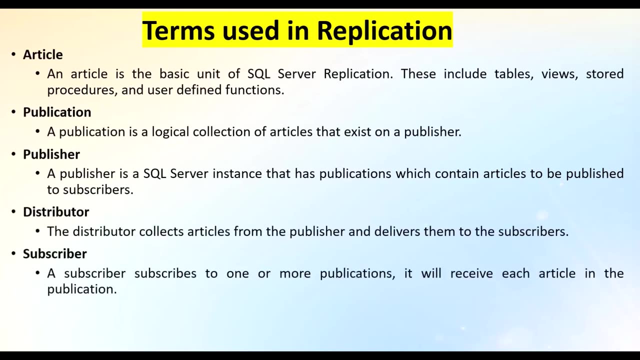 Here in replication we use printing press technology terms like article, publication, publisher, distributor, subscriber and subscription. So in SQL Server replication and article is a basic unit of replication, which include tables, views or stored procedures. Publication is the logical collection of articles or we can say it is a group of articles. 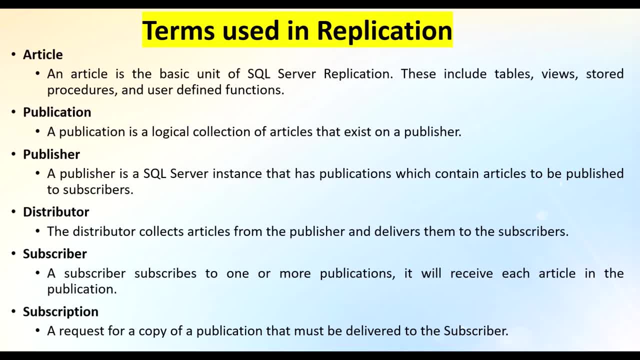 Next publisher. It is a SQL Server instance that contain the publications, So where you are going to create your publication that we call it as a publisher. Next distributor. The distributor collect articles or the publications from the publisher and delivers them to the subscribers. 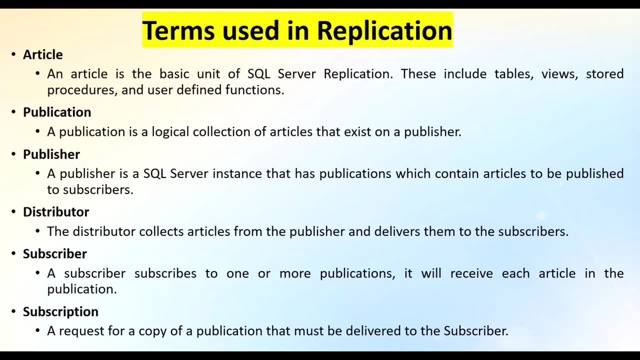 That means it receives and publishes the data, That is, it delivers to the subscribers and a subscriber- A subscriber is a destination or the target who will receive the publication from the publisher via distributor And next subscription. It is a request copy of publication that must be delivered the subscriber. 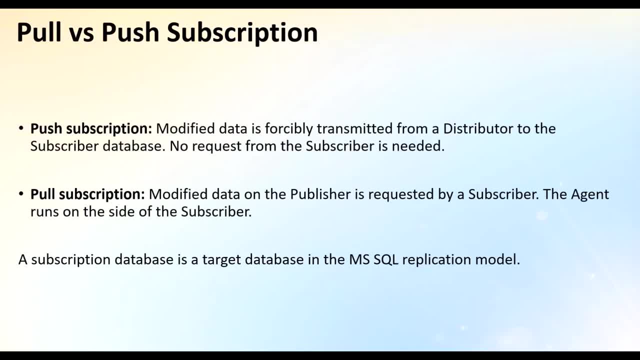 We have Pull subscription and Push subscription. In Push subscription the modification and Gone subscription are the same. Now let us describe what pull subscription is and what Lyndet subscription is. Let us start with Pull subscription. data is forcefully transmitted from distributor to the subscriber database. 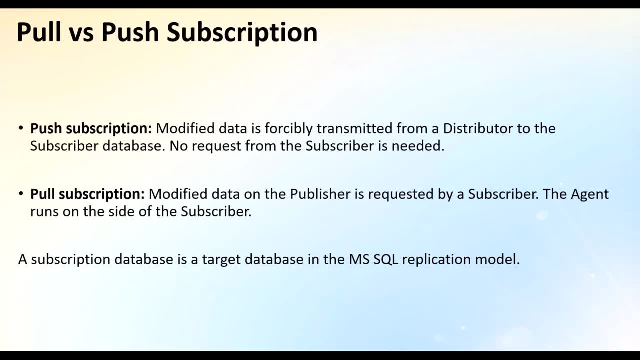 and there is no request from the subscriber is required, whereas input subscription the subscriber has to request for the modified data and the agent will run on the side of the subscriber. so we have different types of agent which we will discuss in each type of the replication in the next coming. 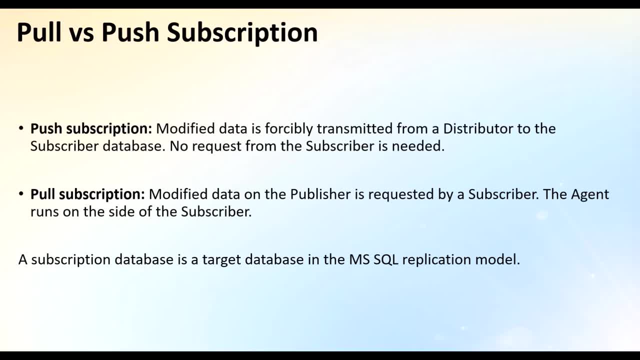 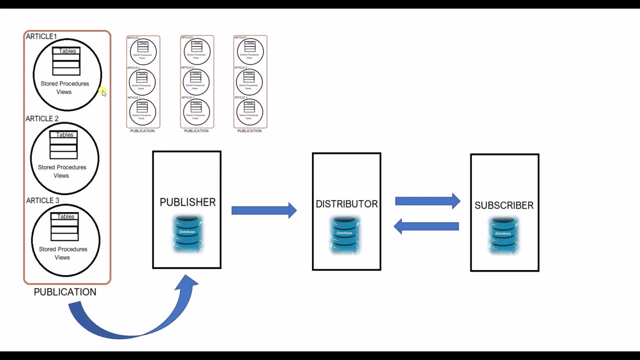 videos. let me show you a simple diagram of articles, publication and publisher. so here you can see the articles. here I have three articles and total four publications, each having three articles in it and, as I said, an article is a group or collection of database objects that can be tables, views or any stored. 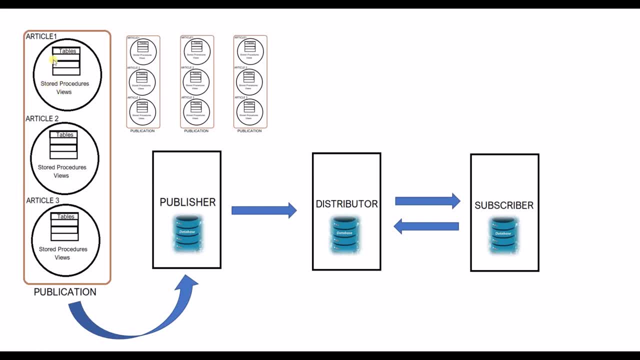 procedures. group of database objects can be called as an article, group of articles can be called as a publication, and these are created at the publisher side, which is the publisher side, which is the publisher side, which is the is a sql server instance and you will have a publisher database here in the publisher. 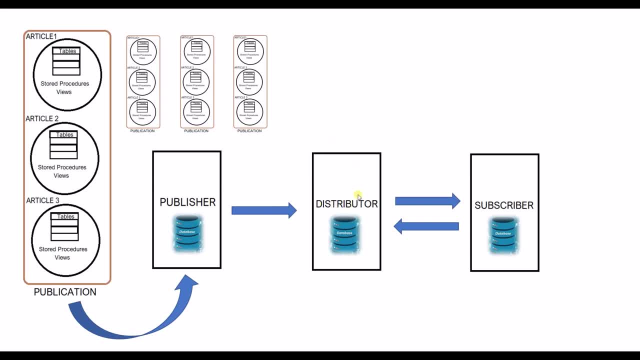 and we have a distributed database here. this can be another sql server instance. similarly, you will have one or more subscribers here and the communication can be bi-directional and unidirectional. depends on the type of replication that you are going to implement. here we can say: 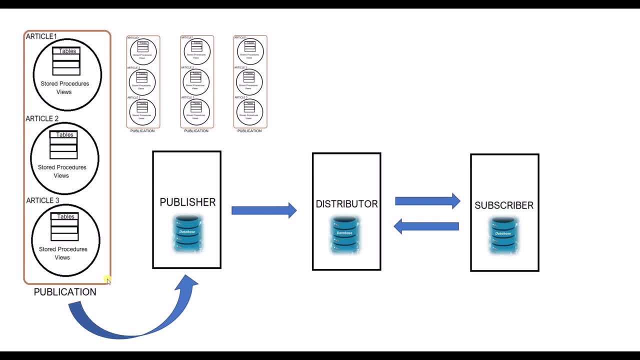 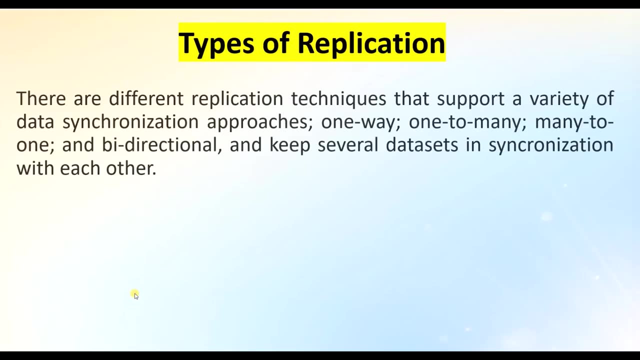 the publisher is the source and the target is the subscriber, and distributor is a mediator which collects information from the publisher and then delivers to the subscriber. okay, so we have total four types of replication, and they are: snapshot replication, transaction replication, merge replication and p2p replication. snapshot replication and transaction replication. 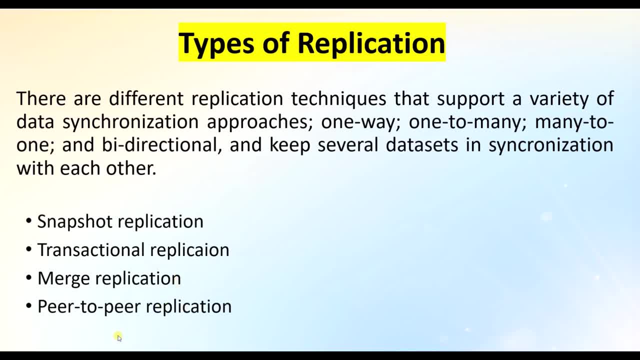 are unidirectional, whereas merge and p2p replication are bi-directional. the most commonly used replication are snapshot replication and transaction replication, so in the coming videos will. we are going to discuss each one in detail, along with the configuration. let me switch to ssms, so here i have two instances. you can see here replication, so this feature will. 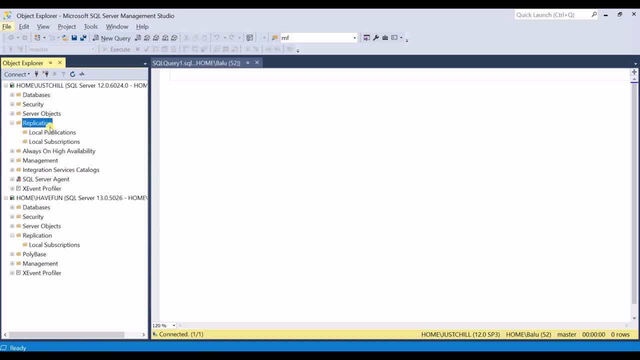 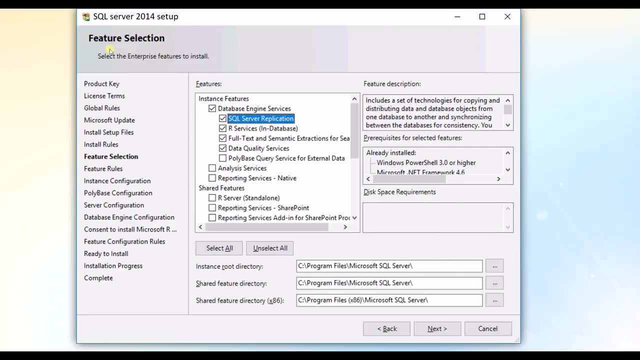 be enabled only if you install this during the sql server installation. i mean you have to take this replication. let me show you the setup file. so here, when you are installing the sql server, at the feature selection pane you need to choose sql server replication. then only the required services will be installed and you will be able to. 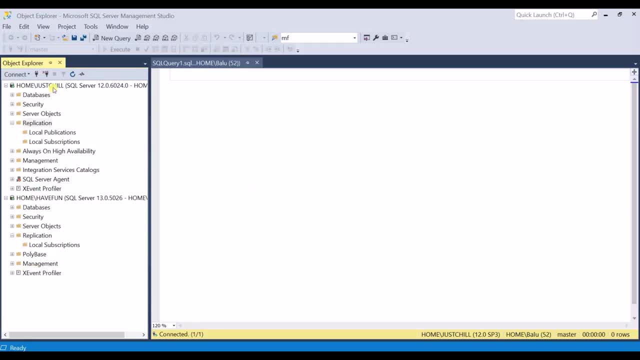 configure replication in sql server. so it is recommended to take separate instances for publisher, distributor and subscriber. so here i have only two. I'll try to install another instance and I'll set up the replication like snapshot or transaction replication in the next coming videos. I hope you have. 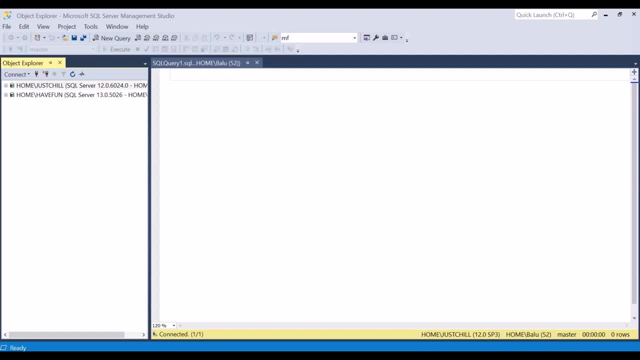 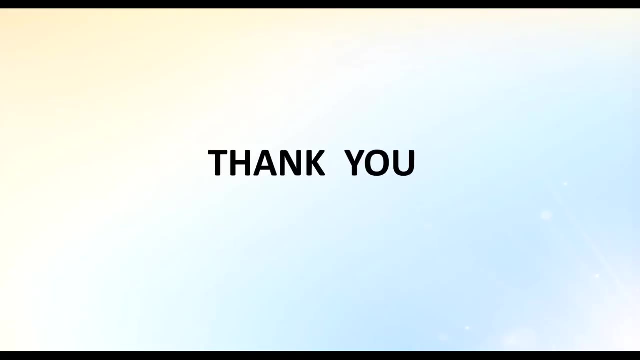 understood the basic concept and terminology of replication. I have already made videos on other high availability technologies. you can find the links in the description. okay, let's meet in part 2, thank you. thank you for watching. if you liked the video, please hit like button. do subscribe and share. match.